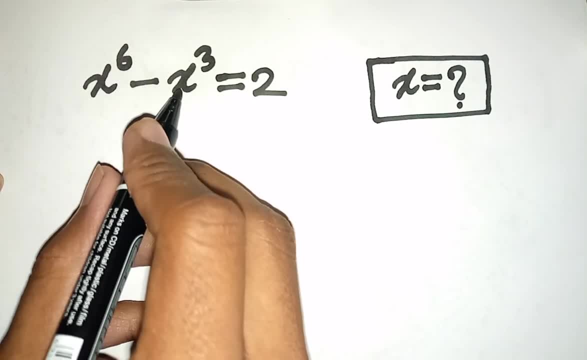 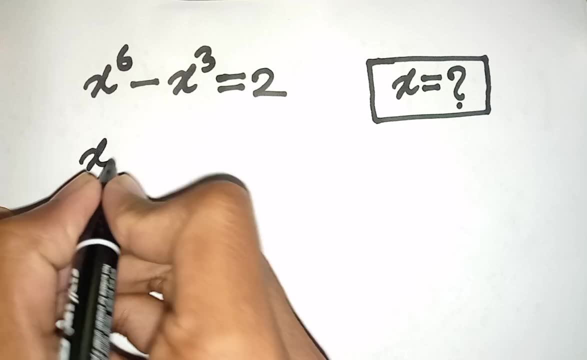 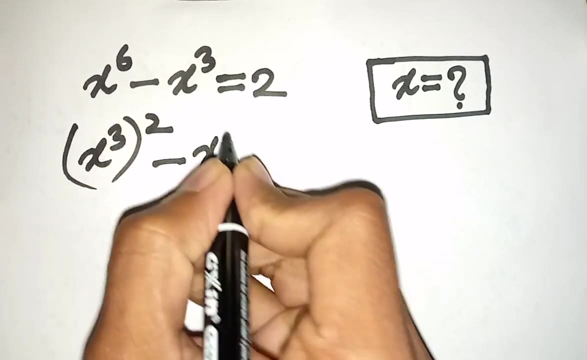 How to solve x power 6 minus x power 3 is equal to 2?. Find the value of x. So we have x power 6 is same as x power 3, bracket power 2.. Then minus x power 3 is equal to 2.. Now we see x power 3,. 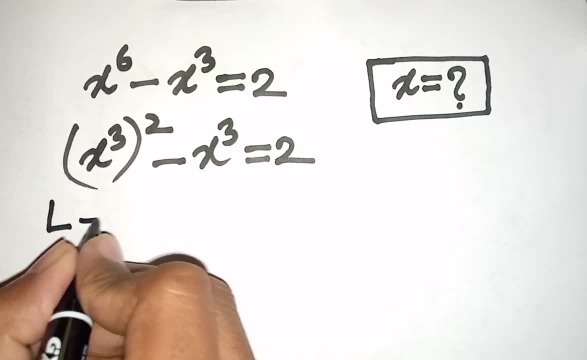 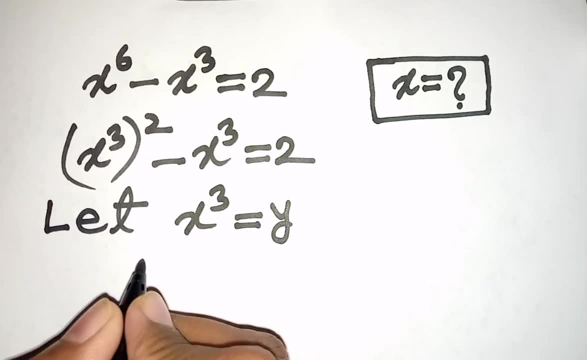 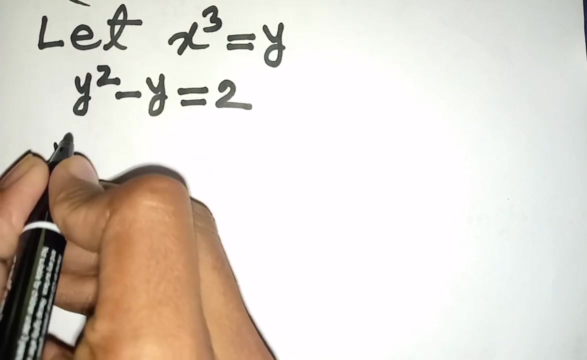 x power 3, both term is same, So let x power 3 is substituted by y, So our equation will be: y square minus y is equal to 2.. Now we can write here: y square minus y, Then plus 2, take to the right. 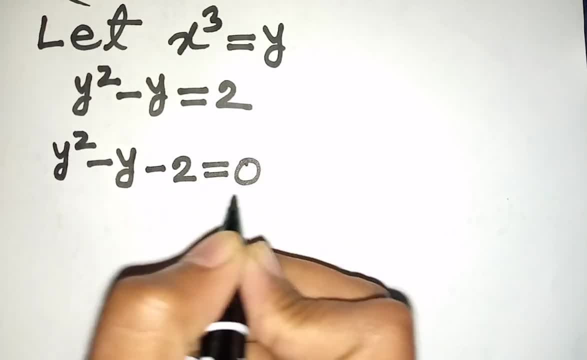 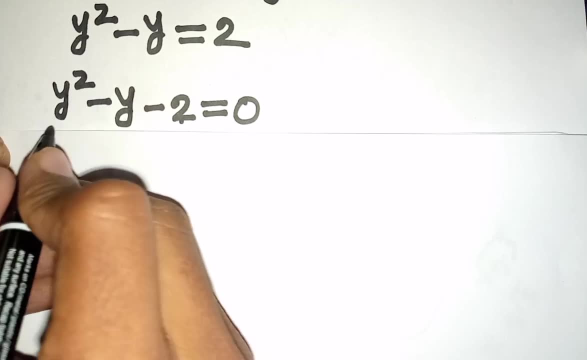 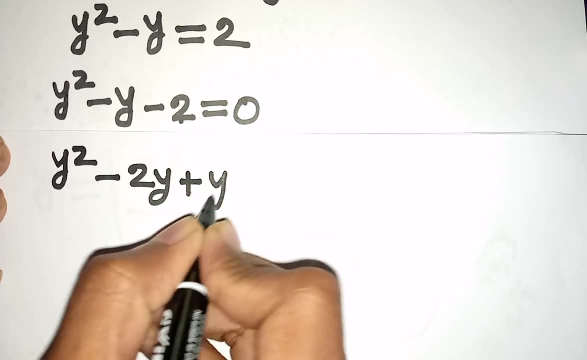 So this will be: minus 2 is equal to 0.. Now we can write here: we can apply quadratic formula or middle term factorization. I just middle term. So we can write here: y square minus y is same as minus 2y plus y. This is middle term factorization. These times these will be same. These times these. 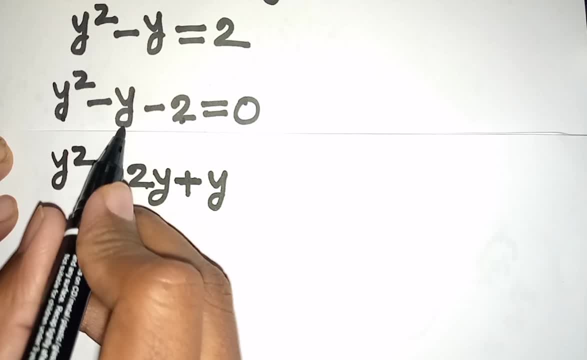 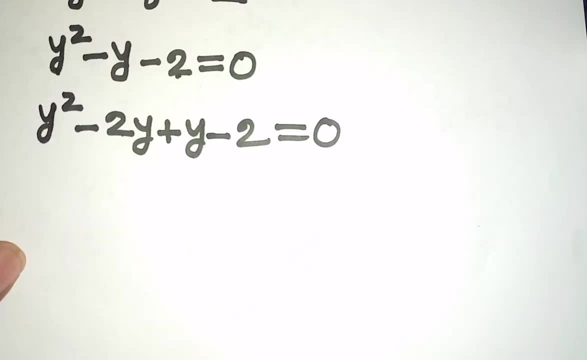 and minus 2y. plus y, That means minus y. So this is middle term factorization. Then minus 2 is equal to 0. Now here we take common. Here y is common, So y is out of the bracket. This divided by this, That means y Minus 2y. divided by plus y, That means minus 2.. 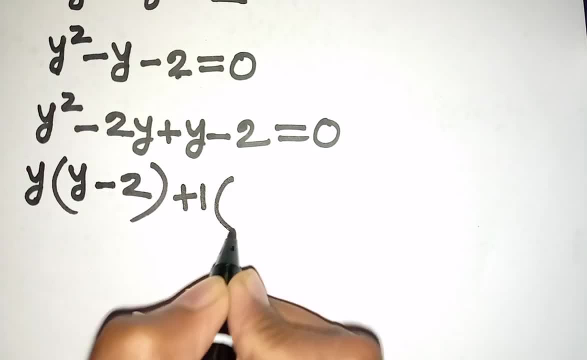 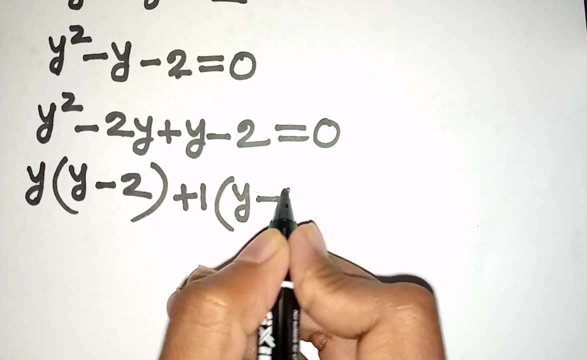 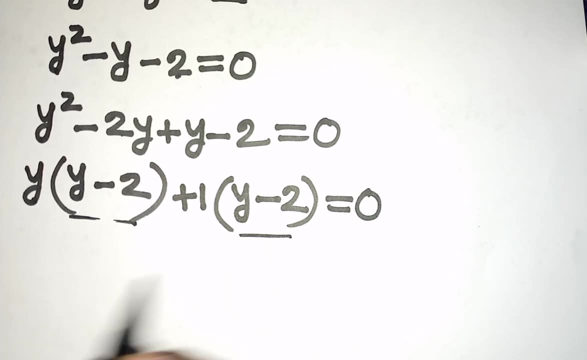 Then here plus 1 is common, So plus 1 is out of the bracket. This divided by this, That means y Minus 2. divided by plus 1. That means minus 2.. Y minus 2 is equal to 0. Now we see y minus 2, y minus 2 is common, So bracket y minus 2 is out of this bracket. 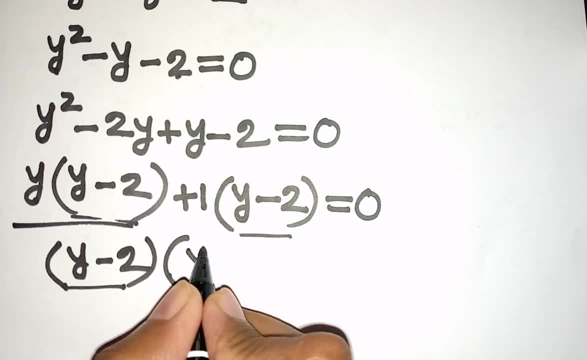 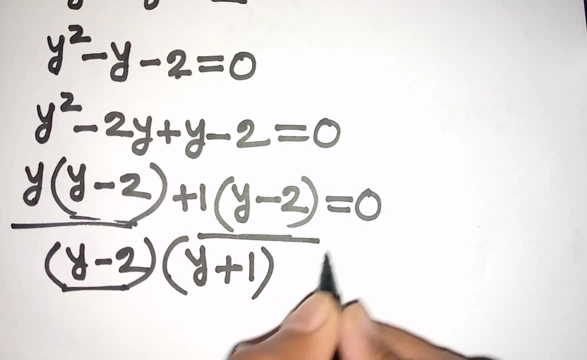 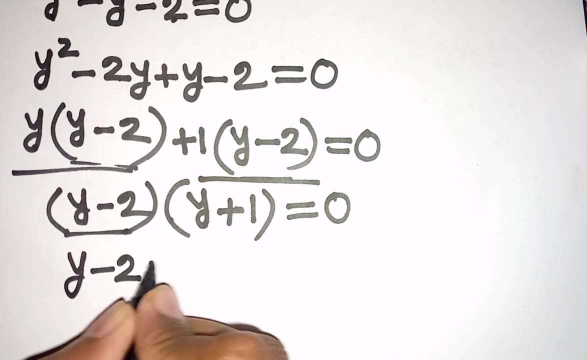 So this divided by this, That means y. Then plus this, divided by this, That means 1 is equal to 0.. Now we can write here: y minus 2.. Y is equal to 0, or y plus 1 is equal to 0.. 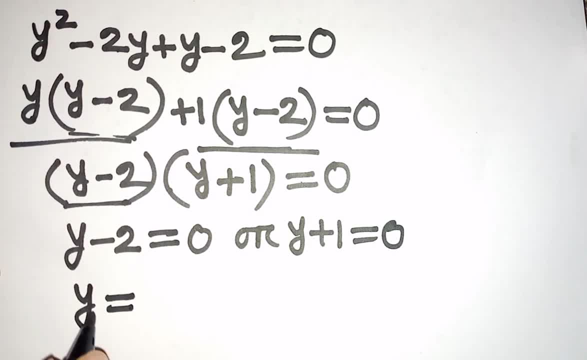 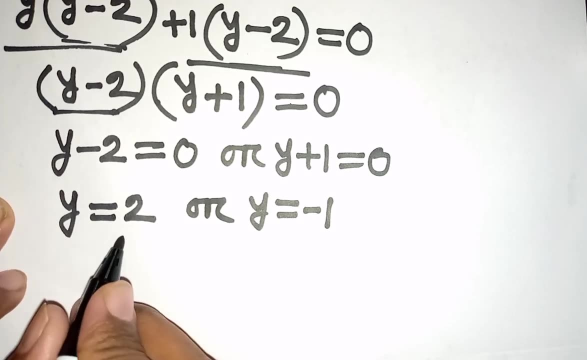 Now we can write here: y is equal to minus 2.. Take to the right side, So this will be plus 2, or y is equal to plus 1. Take to the right side, So this will be minus 1.. Now, here y is equal to 2.. 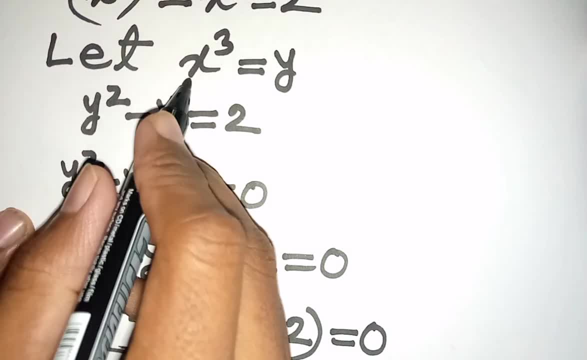 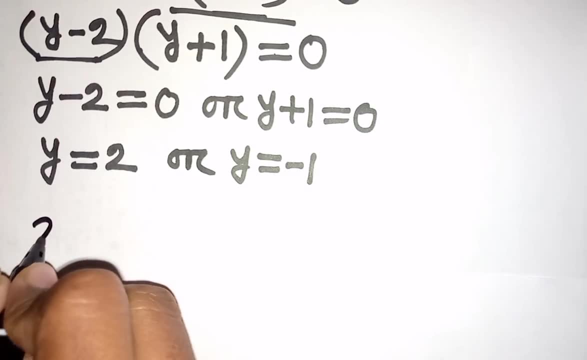 But remember, let x power 3 is substituted by y, So y, that means x power 3.. So y, that means x power 3 is equal to 2, or y, that means x power 3 is equal to minus 1.. 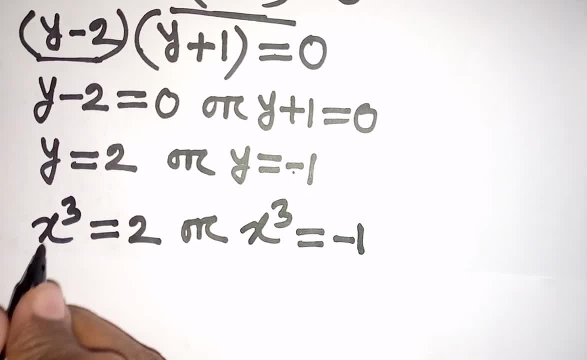 Now we can write here: we have x power, 3 is equal to 2.. Now we take cube root both sides, So cube root of x cube is equal to cube root of 2.. Or here we take cube root both sides, So we can write here: cube root of x cube is equal to 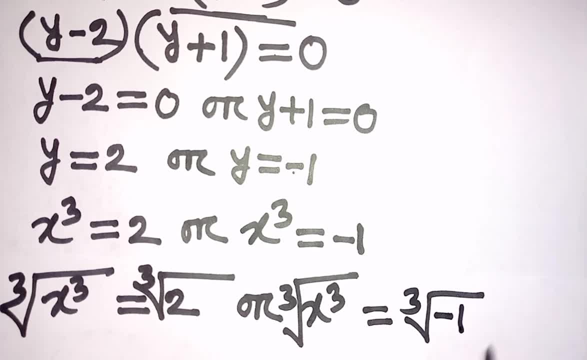 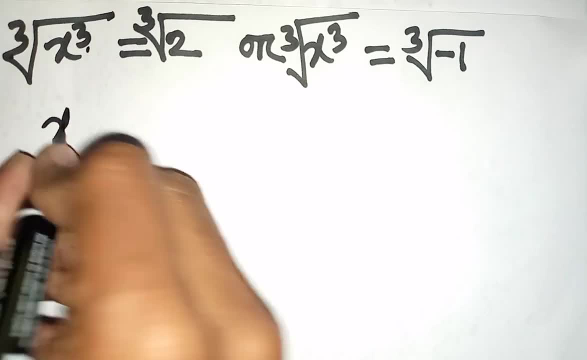 cube root of minus 1.. Now we see this cube root, this power 3 will be cancelled. So here we have x. power 3 is equal to minus 1.. So here x is equal to cube root. 2 is same as 2 power 1 by 3.. 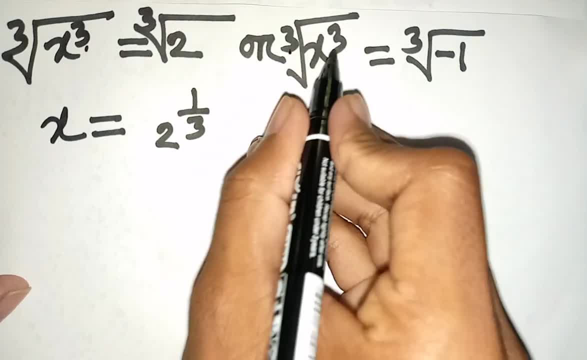 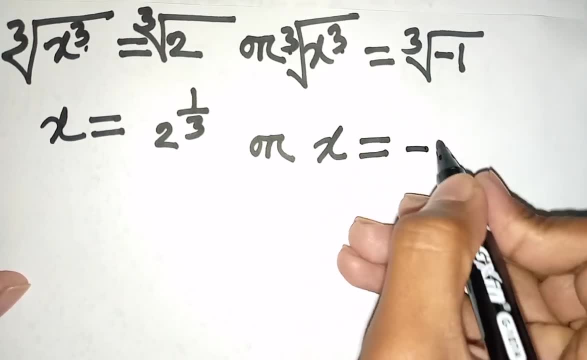 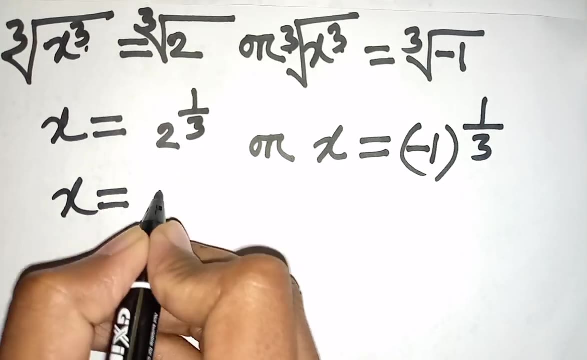 Or we see this cube root. this power 3 will be cancelled. So here: x is equal to cube root, minus 1 is same as minus 1 bracket power 1 by 3.. Now we can write here: x is equal to 2, power 1 by 3. or 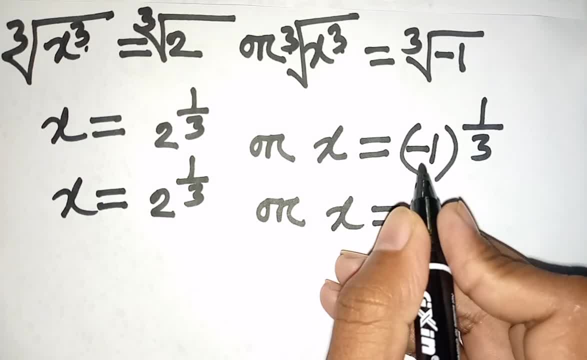 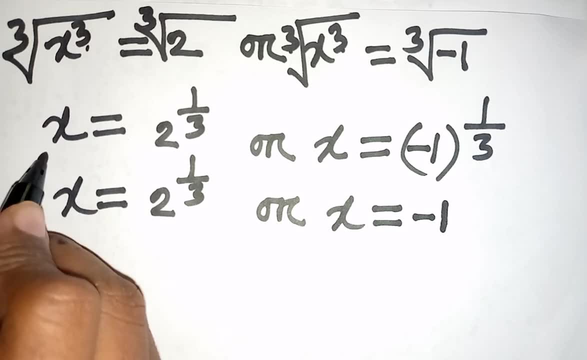 x is equal to minus 1 bracket power 1 by 3.. So here x is equal to minus 1 bracket power 1 by 3 is same as minus 1.. So these are the values of x. x is equal to 2 power 1 by 3, or x is equal to minus 1.. 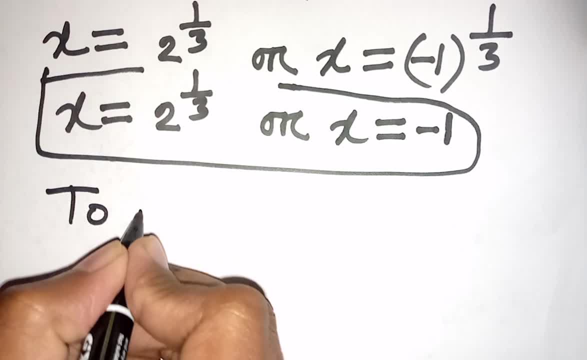 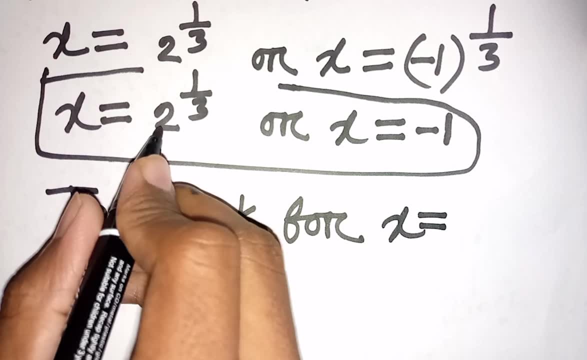 Now to check. to check for: x is equal to 2 power 1 by 3, 2 power 1 by 3.. So we can write here: x is equal to 2 power 1 by 3, or x is equal to minus 1.. 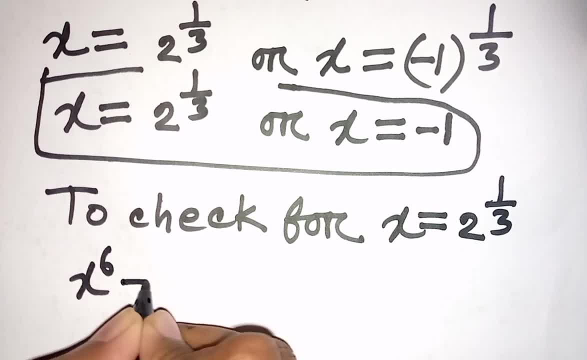 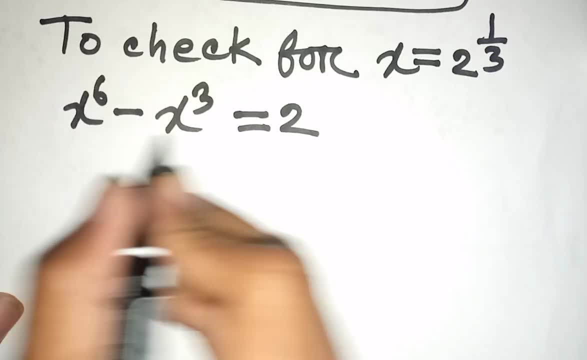 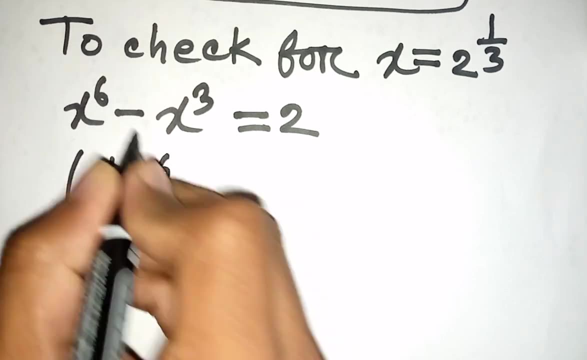 Our equation: x power 6 minus x, power 3 is equal to 2.. Now x, that means 2 power 1 by 3.. So x, that means 2 power 1 by 3. bracket power: 6 minus x, that means 2 power 1 by 3.. So 2 power 1 by 3. 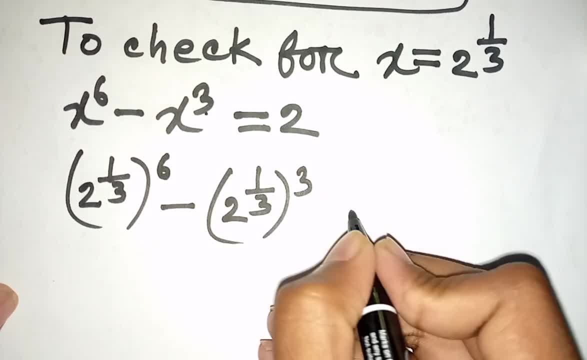 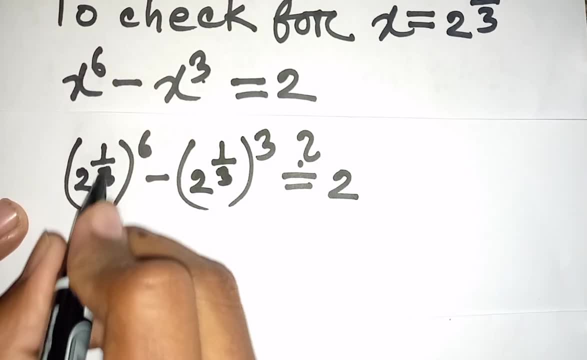 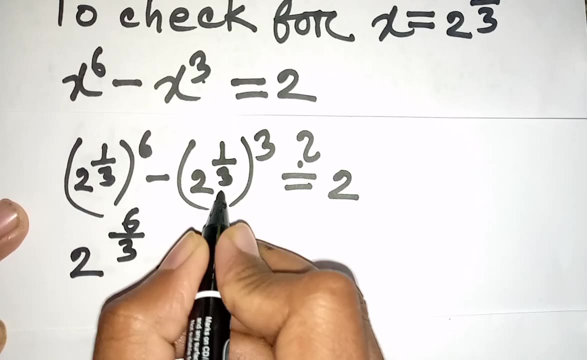 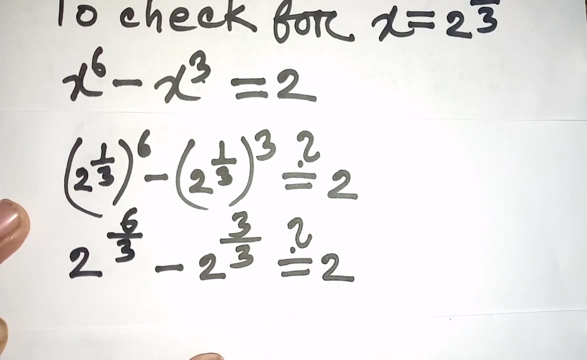 bracket power 3 is equal to 2.. Now we can write here: 2 power 1 by 3 times 6, that means 6 divided by 3 minus 2. power 1 by 3 times 3, that means 3 divided by 3 is equal to 2.. Now we can write here: 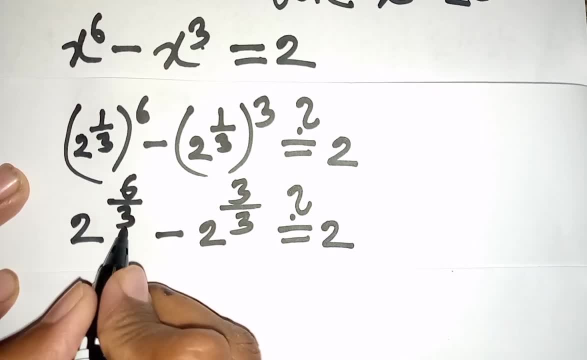 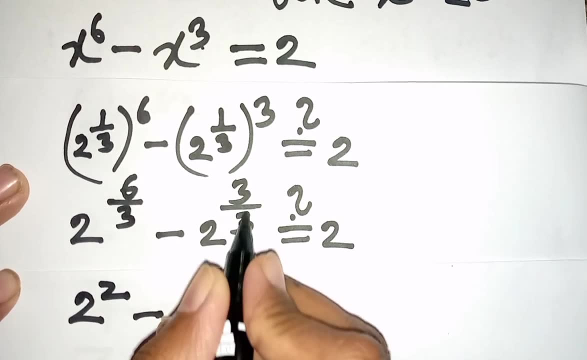 2 power 6. That means 2.. Then minus 2 power 3, divided by 3, that means this: 3. this 3 will be cancelled. So here 2 power 1 is equal to 2.. Now we can write here: 2 power 2, that means 4 minus 2 power 1. that 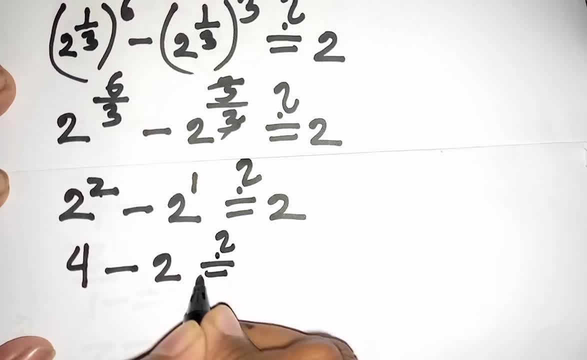 means 2 is equal to 2.. Now we can write here: 4 minus 2, that means 2 is equal to 2.. Now we can write here: 4 minus 2, that means 2 is equal to 2.. Now we can write here: 4 minus 2, that means 2 is. 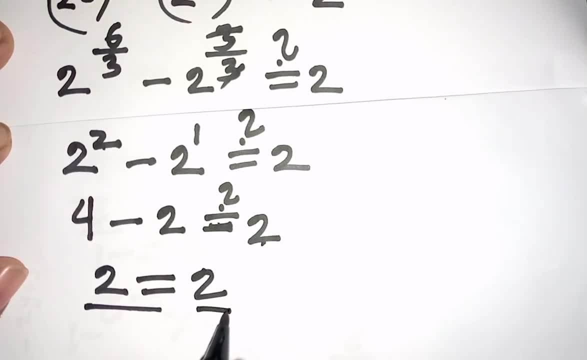 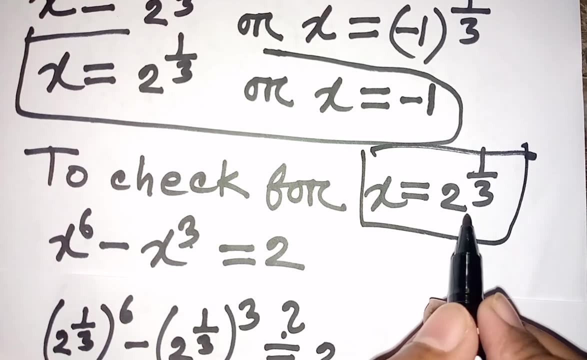 equal to 2.. So 2 is equal to 2.. Left side is equal to right side, So our correct answer will be: x is equal to 2 power 1 by 3.. Now we check for: x is equal to minus 1.. Now to check for x is equal to: 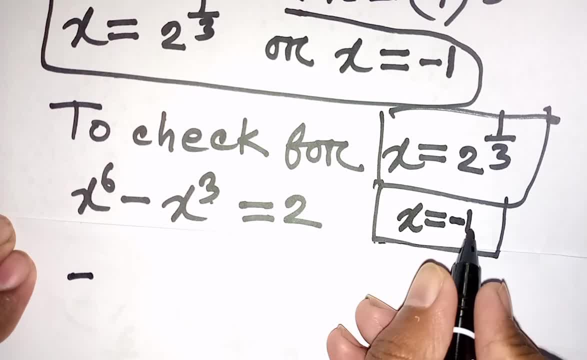 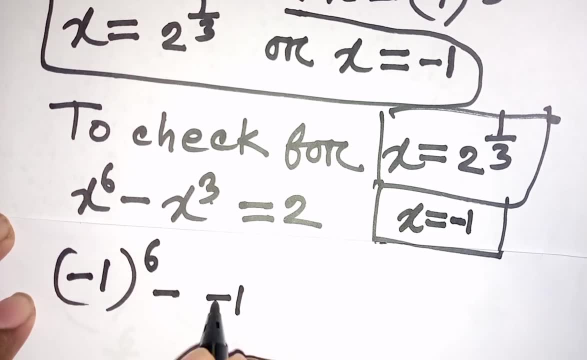 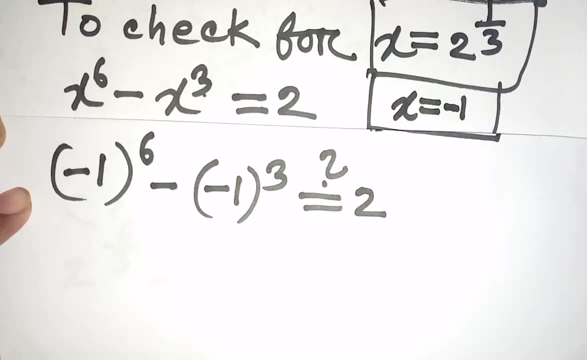 minus 1.. So we can write here: x, that means minus 1 bracket power. 6 minus x, that means minus 1 bracket power, 3. x is equal to 2.. Now we can write here: minus 1 bracket power, 6, that means 1. Then minus bracket. 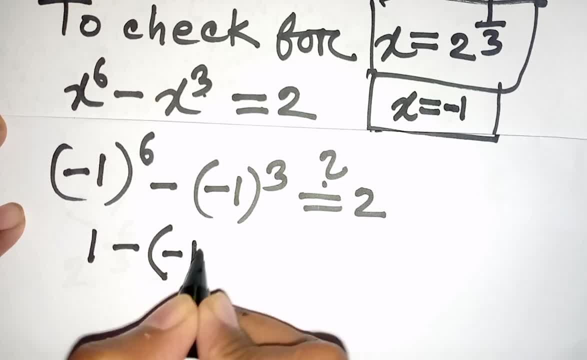 minus 1. power 3, that means minus 1, is equal to here. minus 1 bracket power 3, that means minus 1.. Then is equal to 2.. Now we can write here: 1 minus times minus, it will be plus 1..